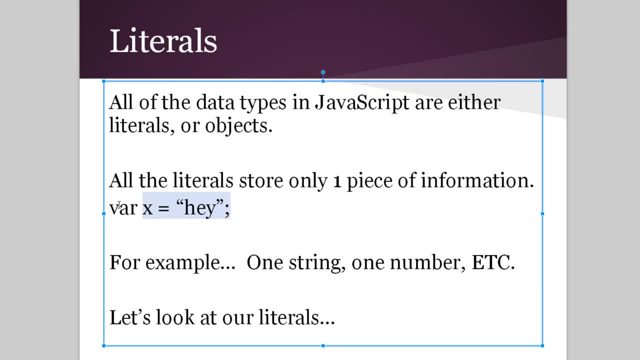 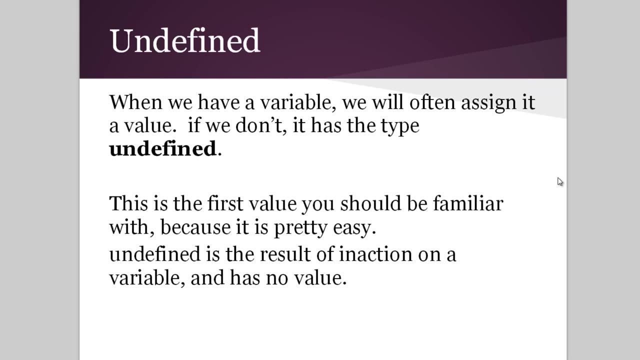 We enclose the string within quotation marks. So this is a literal. We also have objects, but we'll be getting into that as we go through this video. So let's look at our literals. First one is undefined. Basically, that's when we have a variable- and we usually with variables- we assign it a value, But if we don't, it has the type undefined because we haven't given it a value. 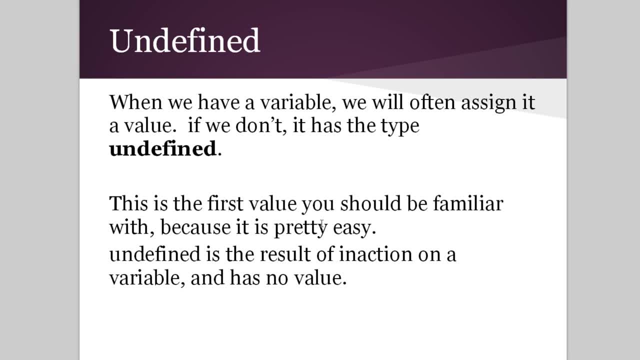 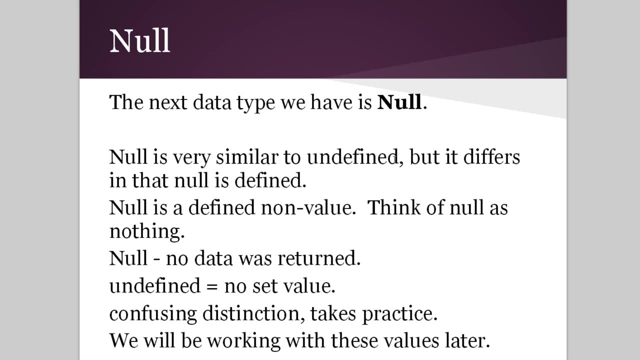 This is the first value you should be familiar with because it's pretty easy to understand. Undefined is the result of inaction on a variable. It has no value, So we assign it a value. So let's look at our literals. has no value. Now the next one, very similar, is null. Null is very similar to. 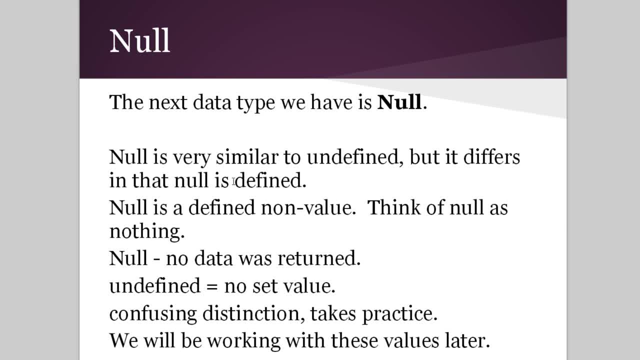 undefined, but it differs in that null is defined. So null is defined. non-value: It's a non-value, but it's defined. Think of null as nothing. So null, basically no data was returned, Undefined, though I guess I should make. 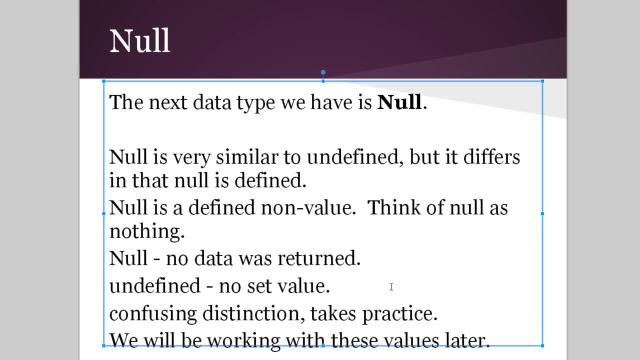 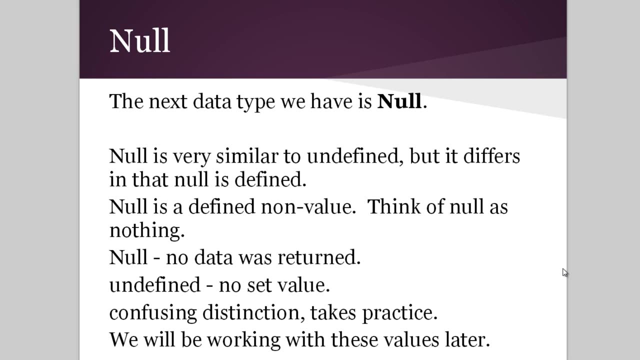 it consistent here has no set value. So when no data was returned, it's null. But undefined is basically saying oh, nothing's been done with this variable Confusing distinction and it takes practice to understand. but we will be working with both of these later as we go on with our actual scripting, and so 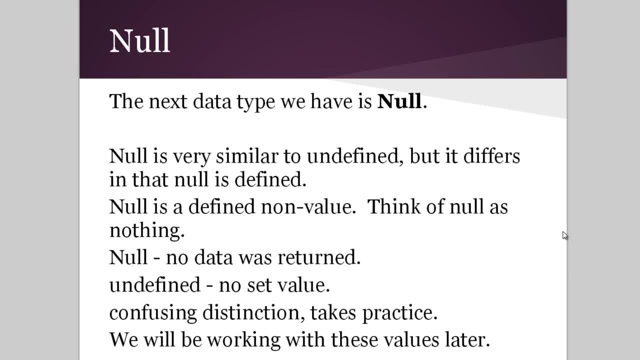 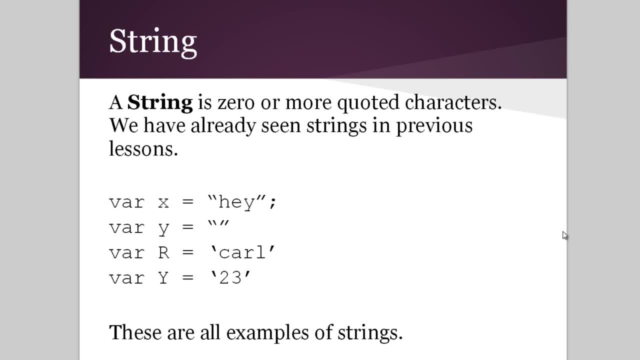 forth. So basically, two values: undefined and null are two. you should be familiar with and understand the distinction between the two. We also have other values, such as string. A string is zero or more quoted characters. We have already seen this in previous lessons, but if you're. 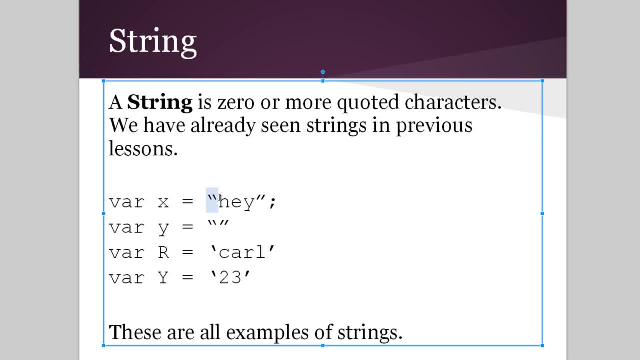 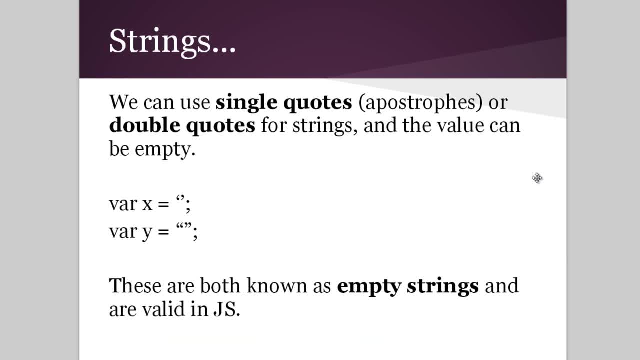 all examples of strings. We can use single quotes, apostrophes, which are also known as apostrophes, or double quotes for strings, And the values can be empty. So these are both empty strings. That's the term you should know, And they're valid in JavaScript. So these are correct You. 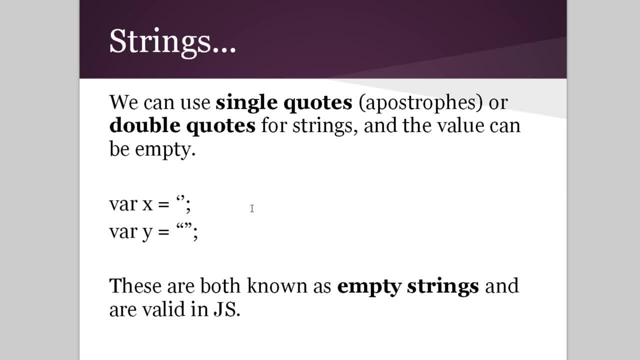 can use these And, once again, an empty string is different than null or undefined. So that's another thing you need to be familiar with. We have null, undefined strings, But within strings we have empty strings, which you may confuse with null or undefined. 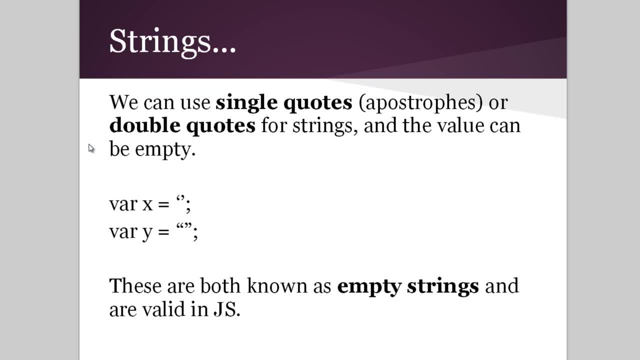 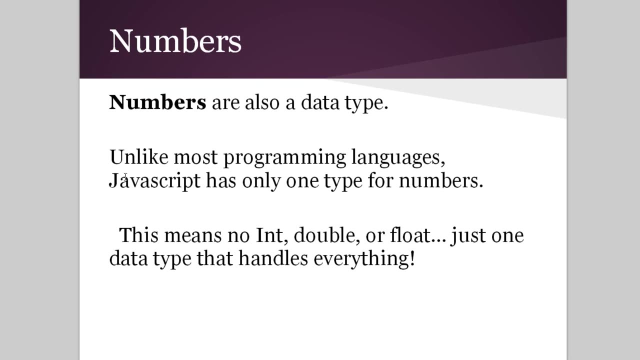 Just be sure to know that there's three data types so far: Strings, null and undefined. And as you go on in your JavaScripting, programming, JavaScripting- it'll start to make more sense. Numbers are also a data type. Unlike most programming languages, JavaScript has. 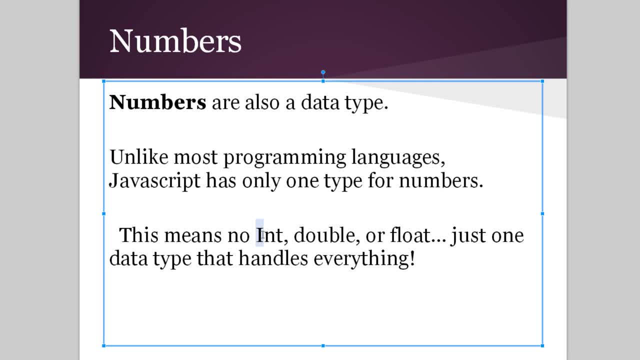 only one type for numbers. That means we don't have to worry about int, int, int, int, int, int, double or float. Just one data type that handles everything which can be useful, And obviously there may be some downsides to that, So here are some. 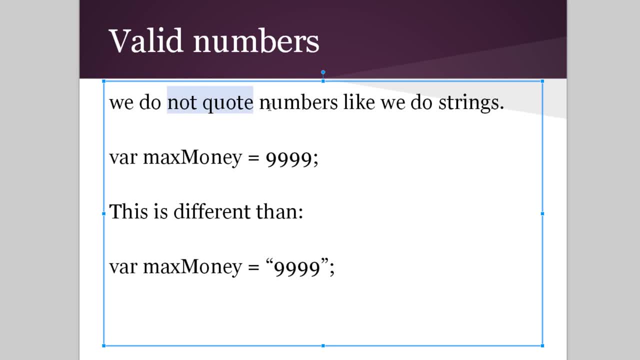 valid numbers. We do not quote numbers like we do strings, So you can see there's no quotation marks right here. We just put the number. That is different than with the quotation marks. So this down here is a string, This up here is a. 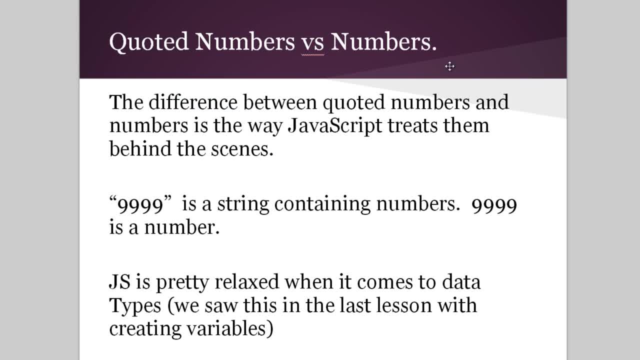 number. So what's the difference? The difference between quoted numbers and numbers is the way JavaScript treats them behind the scene. This is a string containing numbers. 9999 is just a number, So those will work differently in JavaScript And, to be honest, JavaScript. 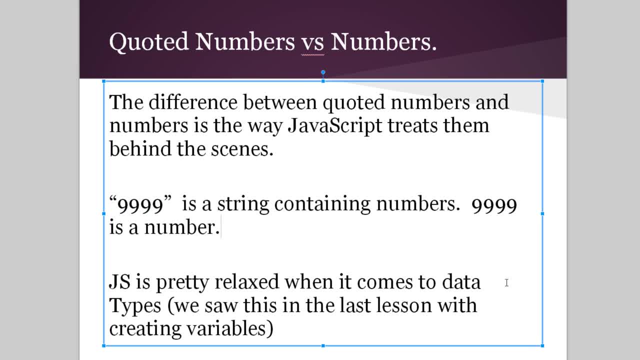 is pretty relaxed when it comes to data types. So we saw this in the last lesson with creating variables. So this means occasionally we may get some conversions between types, So we may think we have a number, but we actually have a string. 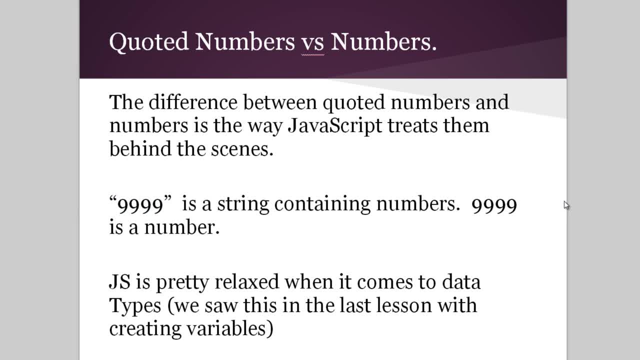 So that can be a downside to JavaScript, when people don't understand how JavaScript works with their data types. And then we get a string rather than a number, which is to be expected. So, for example, if we add a number and a string, it's going to convert the value to a string. 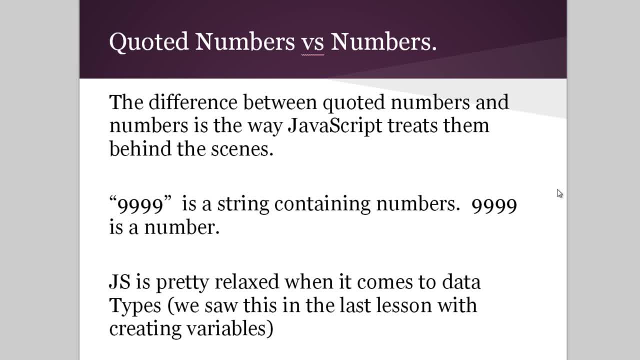 So that's something you need to understand with JavaScript. You have to really understand how JavaScript works with its variables and the data types to understand how to get a specific value and get the correct value, And we'll be going over that in upcoming videos. 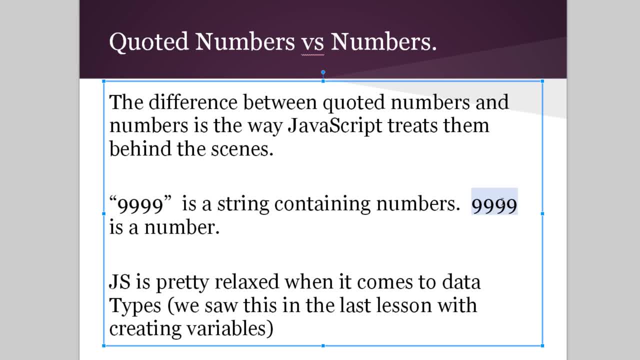 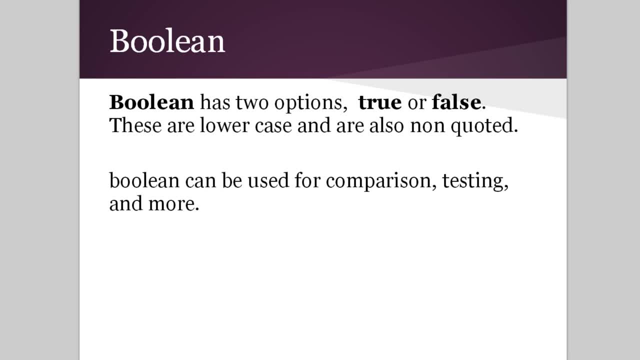 Just understand that these are different. The next data type is Boolean. Boolean has two options: true or false. These are lowercase and are also non-quoted, So this is not Boolean, This is a string. just like that is a string and not a number data type. 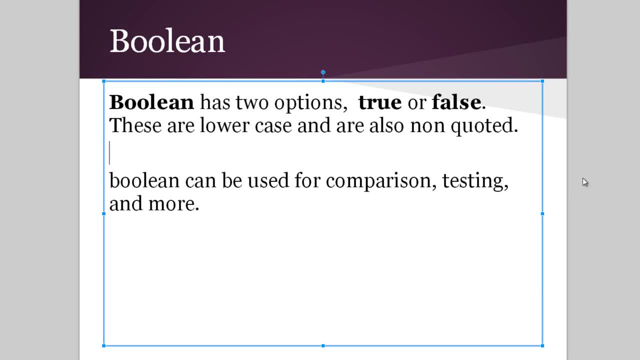 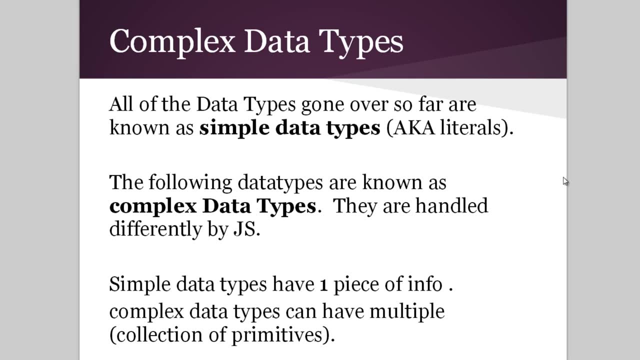 Boolean can be used for comparison, testing and more. All right, so now we're getting into what's known as complex data types. So when we were at the beginning, we said there was two groups, Basically: literals and objects. So far we just went over all of the literals in JavaScript. They are known. 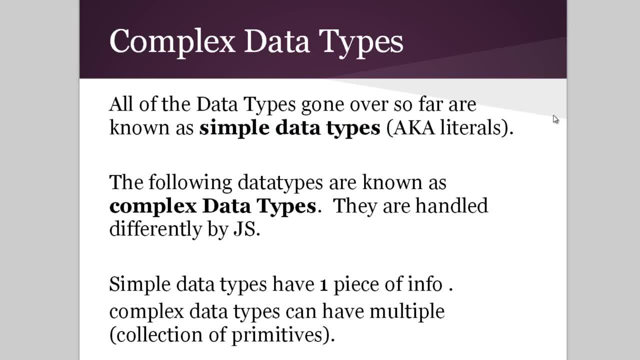 as simple data types because they only store one piece of information. The following data types are known as complex data types. They are handled differently by JavaScript. Simple data types have one piece of info. Complex data types can have multiple, basically a collection of primitives. 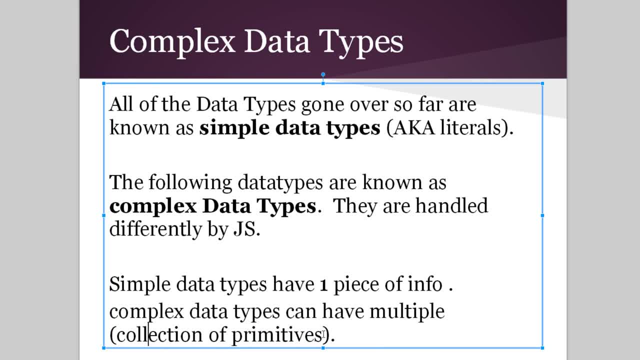 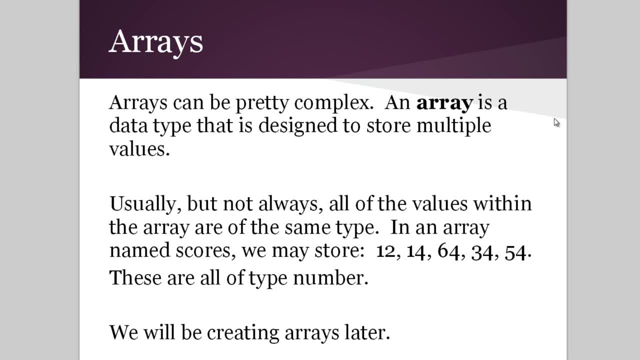 Which I don't even know, if I mentioned what that is. Basically, primitives are all of the literals, So an example of one of these complex data types is an array. This is an object in JavaScript that is designed to store multiple values. Usually when we use arrays, but not always, 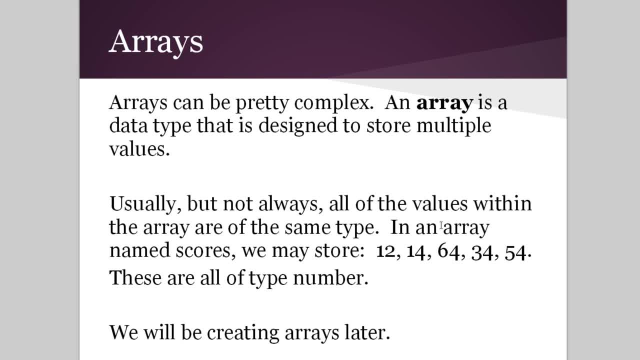 all of the values within the array are of the same type. So in an array named scores we may store 12,, 14,, 64,, 34,, 54. These are all of type number. We will be creating arrays later. 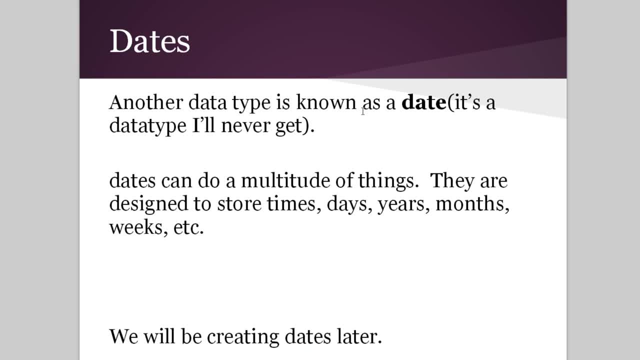 Dates. this is another important object in JavaScript you may want to know about. It's basically, yeah, dates can do multiple multitude of things. They are designed to store times: days, years, months, weeks and so forth. We will be creating dates later. 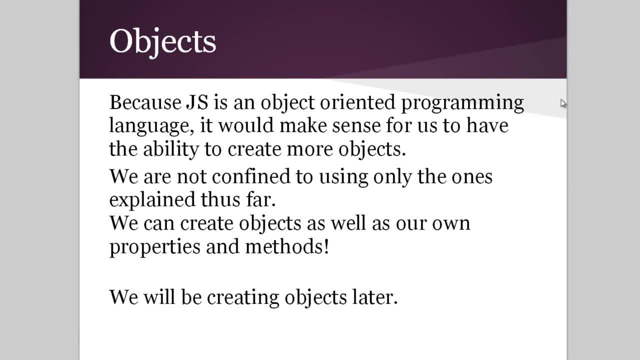 Basically- I'm just giving you an introduction- Objects. because JavaScript is an object-oriented programming language, it would make sense for us to have the ability to create more objects, So we're not just limited to the ones that are already defined, such as dates, date objects or array objects. We can 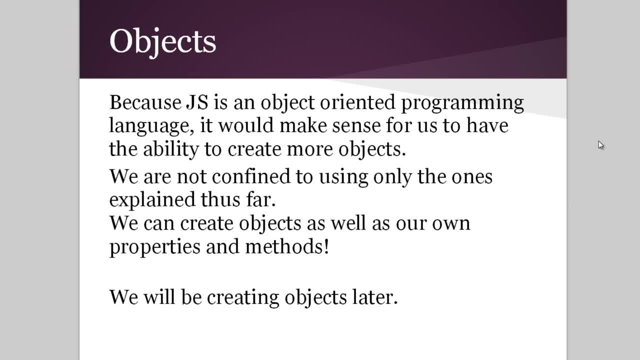 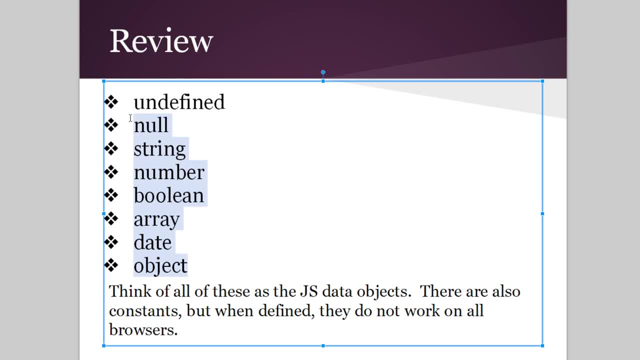 create our own, and we will be doing this as we go farther in our video lessons. So, as a review, here are all of the data types I talked about. These ones are our simple or literals. These ones are objects which we'll be getting into. 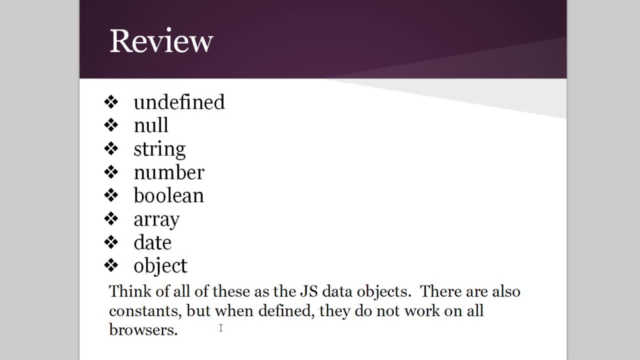 this in comparison in future videos. Sorry, I keep referring to future videos but I can't explain everything at once. It would be impossible. But think of all of these as the basic JavaScript data types or objects. I meant to put types here. 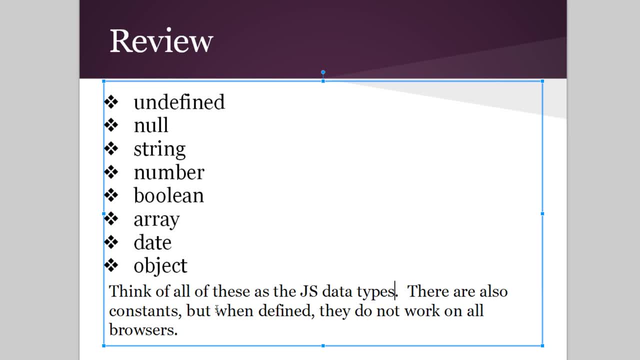 Okay, There are also constants, but when defined, they do not work on all browsers, so we're not even going to talk about those right now. But, yeah, that's basically all of the data types you should be familiar with, and you will be. 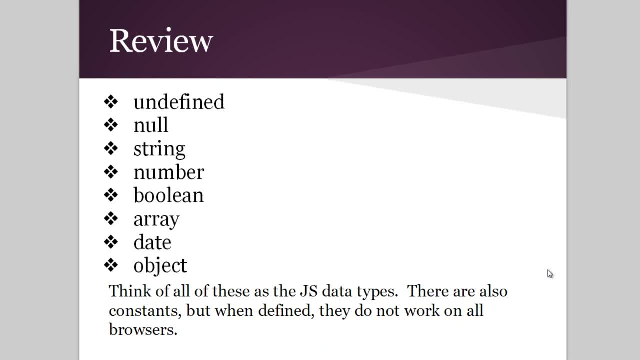 understanding these in a better way as we go on in our JavaScript tutorial series. So thank you for sticking with this far. Hopefully this all makes sense, and I'm trying to give an understanding of how JavaScript works rather than just talking about oh. to define a string, you use single quotes or double quotes- blah.